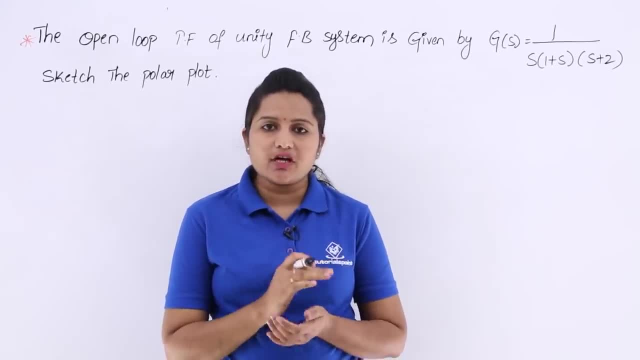 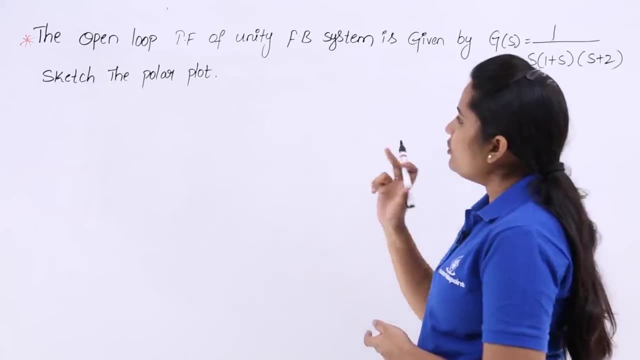 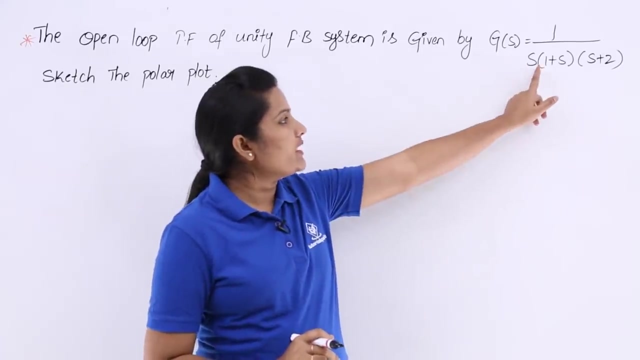 In this video we are going to plot a polar plot by using a open loop transfer function, given. You can observe this problem here. The open loop transfer function of unity feedback system is given by g of s is equivalent to 1 by s, into 1 plus s, into s plus 2.. This is the open loop. 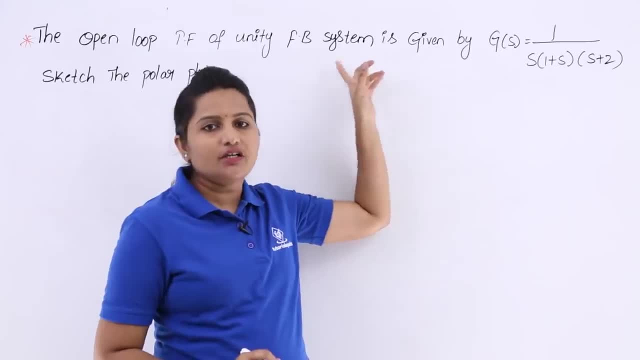 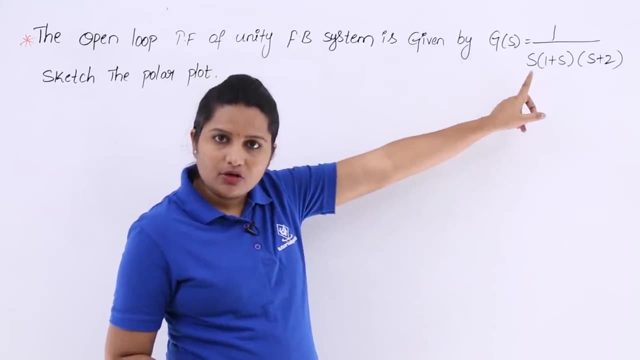 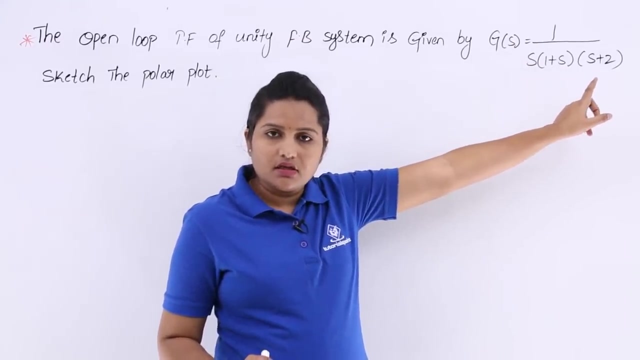 transfer function of a closed loop system which is having unity feedback. That is why I have taken g of s. So if the description is open loop transfer function of a closed loop system, then definitely you will get g of s into h of s here. Why I am having only g of s here. This is: 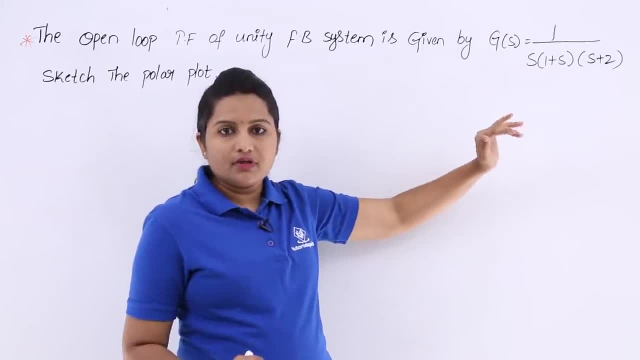 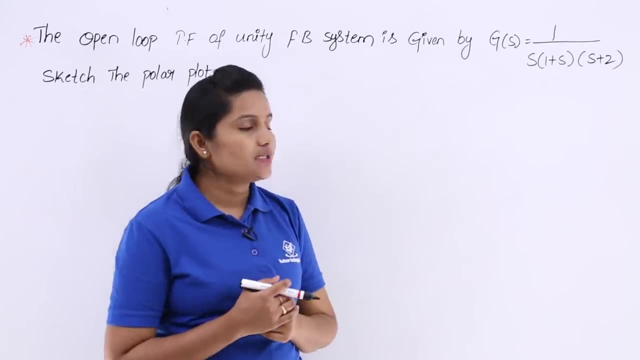 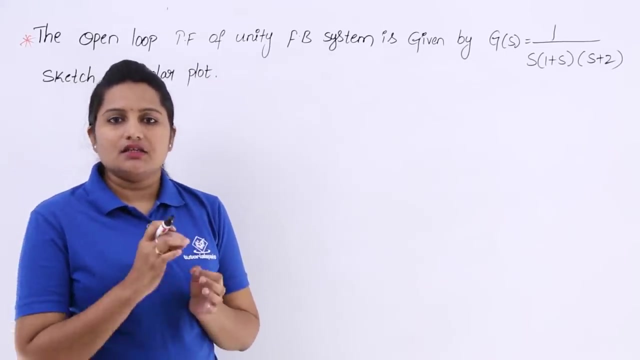 open loop transfer function of a unity feedback closed loop system is: g of s is equivalent to 1 by s into 1 plus s, into s plus 2.. Sketch the polar plot. So first of all we need to consider the first point is the transfer function, the given transfer. 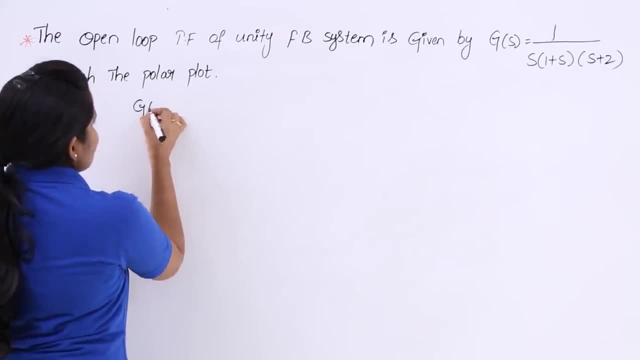 function. I am going to consider my given transfer function. g of s is equivalent to 1 by s into 1 plus s into s plus 2 or s plus 1 into s plus 2. you can consider Now here: substitute: s is equivalent to j omega. If I substituted, s is equivalent to j omega. 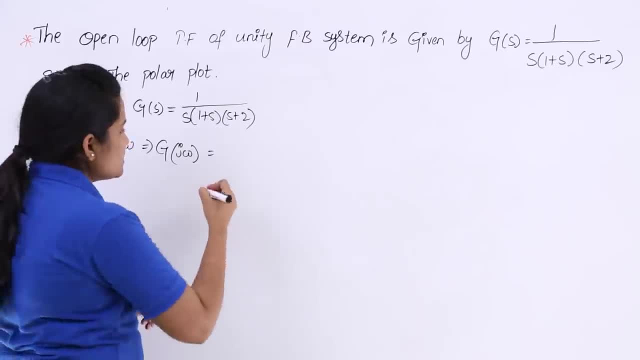 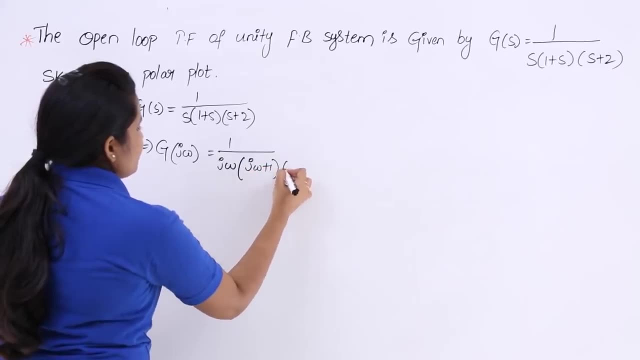 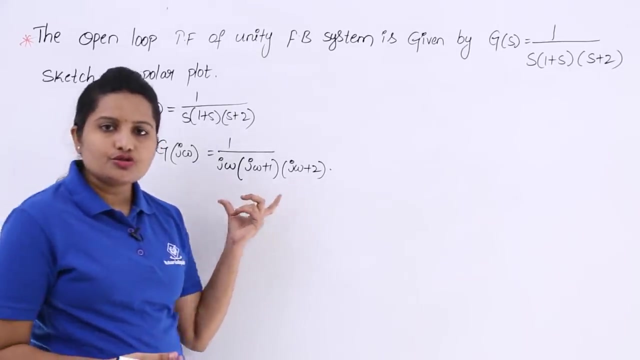 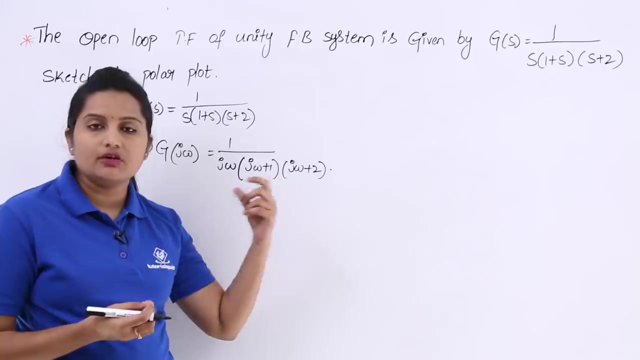 then this open loop transfer function will turns like this: So 1 by j omega into j omega plus 1, j omega plus 2.. So like this we will get Now here to draw any polar plot. we need magnitude and phase of the open loop transfer function. Now I am going to calculate the. 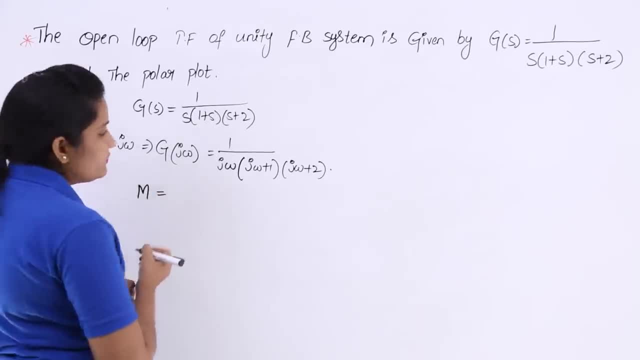 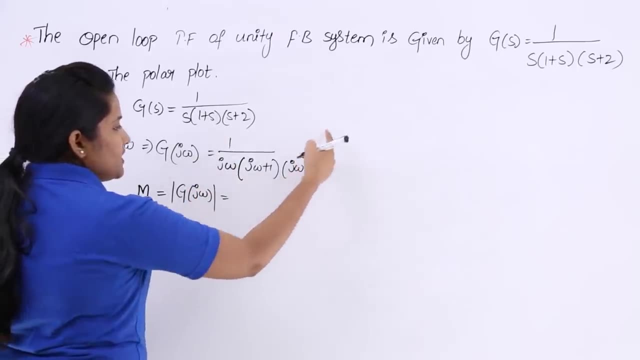 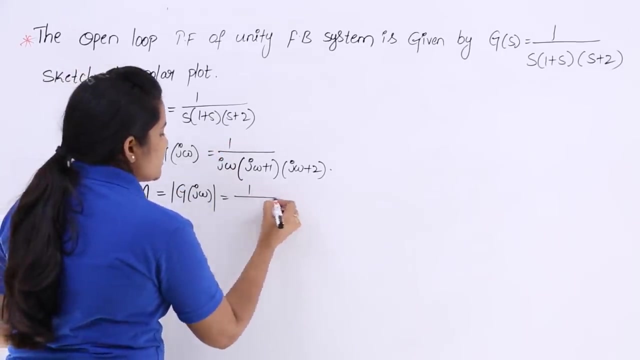 magnitude. magnitude is equivalent to: So to get the magnitude we need to consider modulus of g of j, omega. So the modulus of this term is equivalent to So 1 by modulus of j omega, 1 by modulus of. 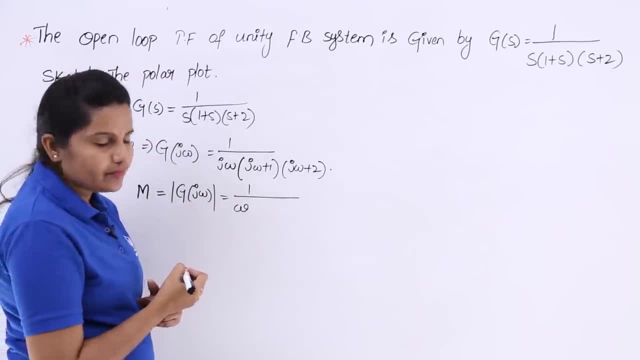 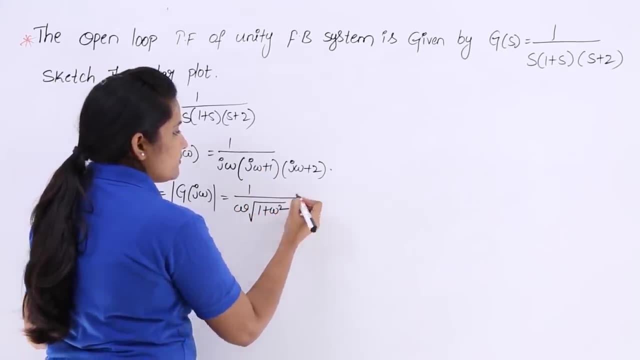 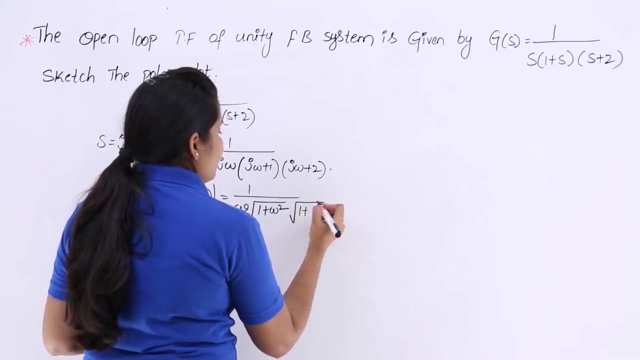 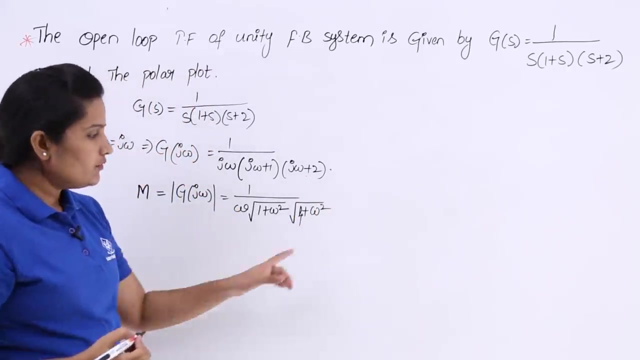 j omega means that is equivalent to omega. So here 1 by j omega plus 1. for this the modulus is 1 plus omega square. For this term that means 1 by j omega plus 2. So for this the modulus is 1 by 2 plus here 2 square. that means 4 plus omega square 4. 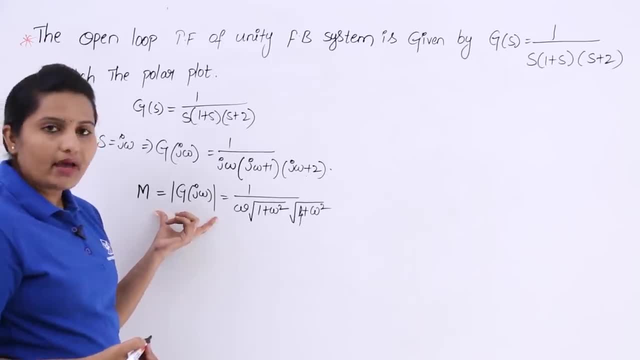 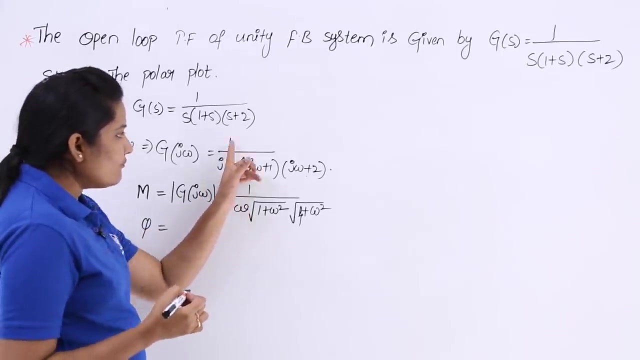 plus omega square. So now here, this is the magnitude of the given open loop transfer function. So now, like this, we need to find out the phase of the open loop transfer function, To find out phase phi. so here, if you observe for this, 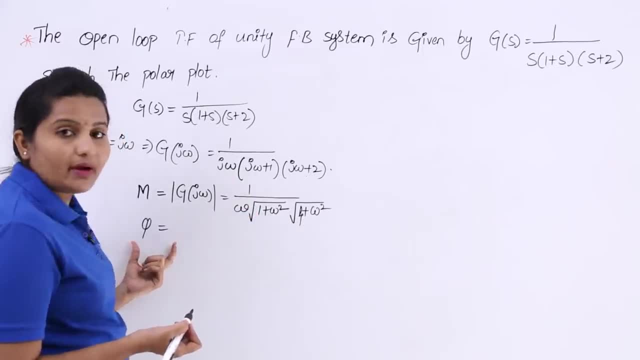 term 1 by j omega. So now you observe this standard magnetic field And we will do it So twice Knight, And then negative square, square. So if you get the speed of the sewn, the phase angle will be minus 90 degrees because you are having j omega term in denominator. 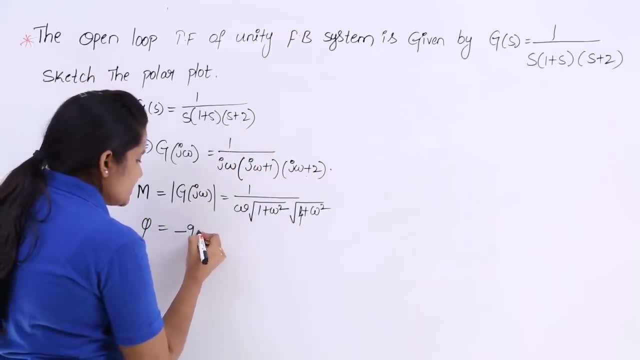 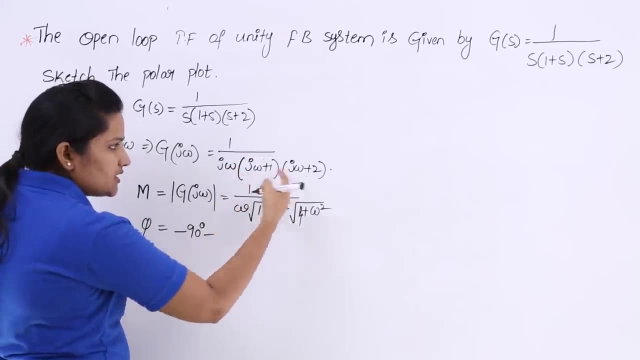 So related to this term, the phase angle is minus 90 degrees. So here 1 by j, omega plus 1. for this the phase angle is. all the terms are in denominator. that is why I am taking minus for phase angle. So minus tan inverse b by a will be the angle phase angle. So here this is b. 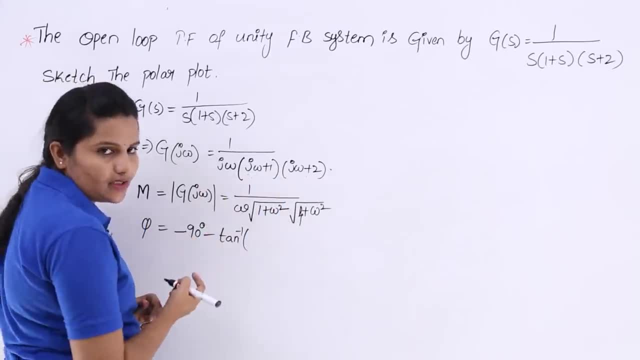 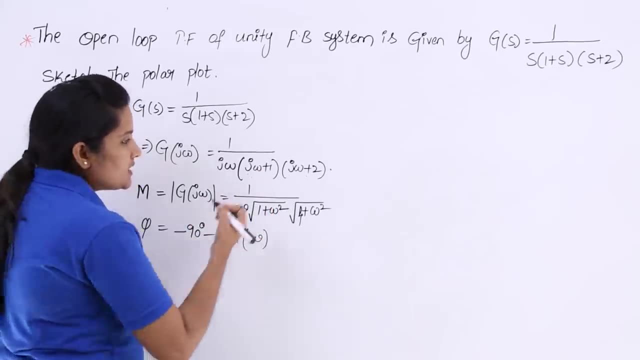 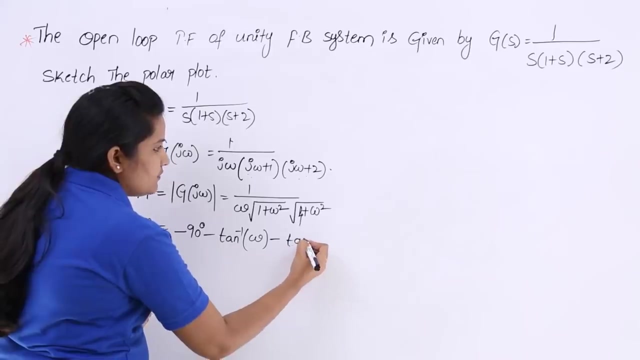 and this is a. I am considering because a plus jb format. So if you want to calculate phase angle, tan inverse b by a, that means omega by 1.. Similarly here minus, as this term is also in denominator. So minus tan inverse, again b by a, means omega by 2.. So this is phase angle and 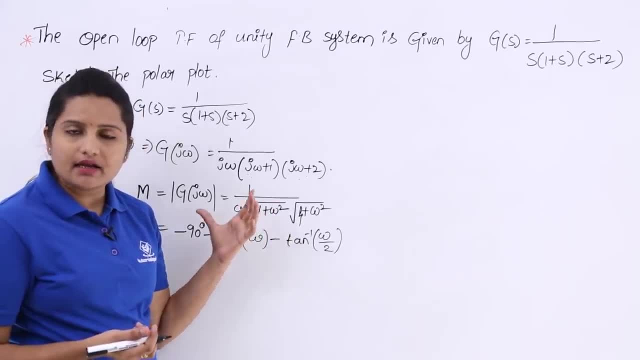 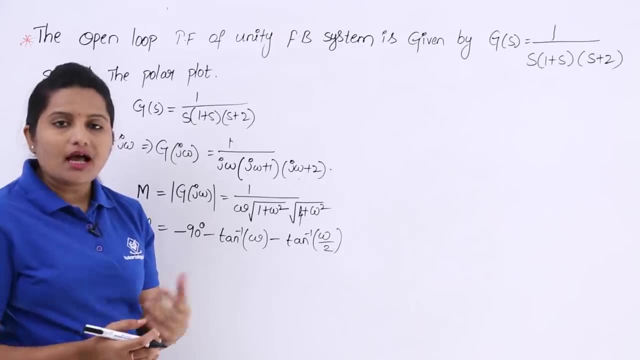 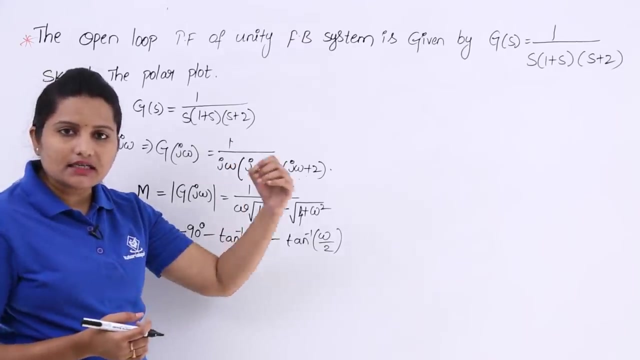 this is magnitude. I got my phase angle and I got my magnitude for the given open loop transfer. To get my polar plot I need to have values at omega is equivalent to 0, as well as omega is equivalent to infinity. At starting value of omega, what will be the values of magnitude and 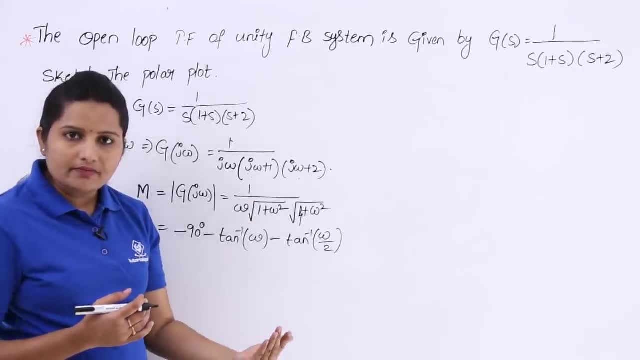 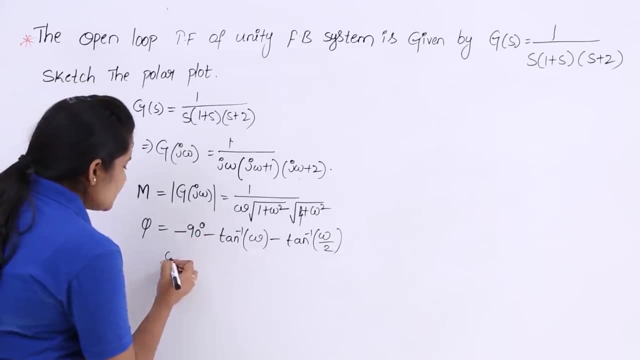 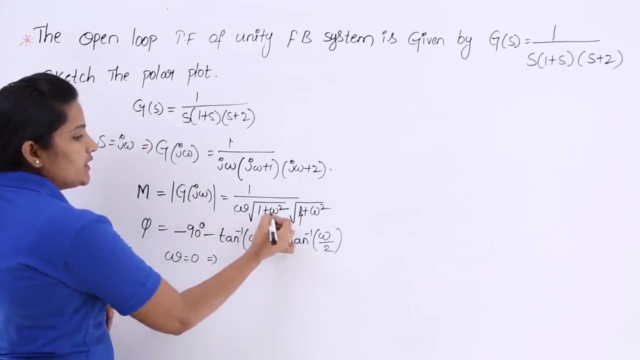 phase I need to observe At ending value of omega. then also I need to observe what is the magnitude and phase. So here I am considering: omega is equivalent to 0. When omega is equivalent to 0, the magnitude is 0. into anything, 0, 1 by 0, infinity. Infinity is magnitude and phase coming. 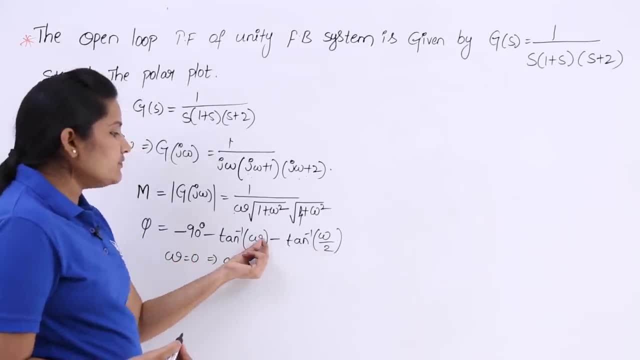 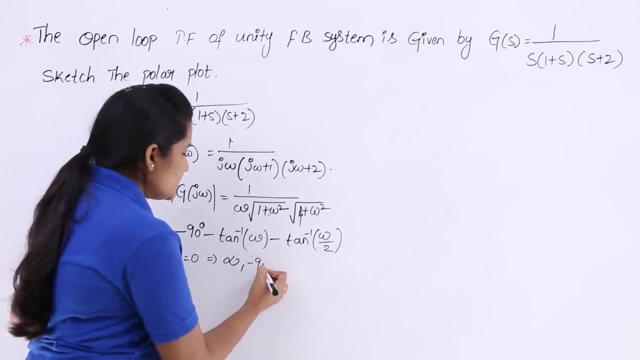 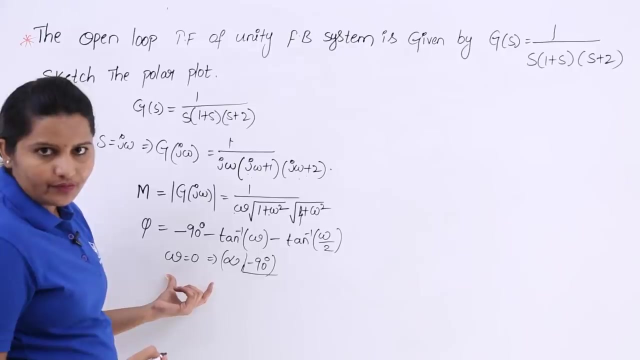 to phase when omega is equivalent to 0- tan inverse 0- tan inverse 0 minus 90 degrees minus 0 minus 0. So I am having minus 90 degrees. So this is magnitude and phase combination, for omega is equivalent to 0.. Now omega is equivalent to infinity. 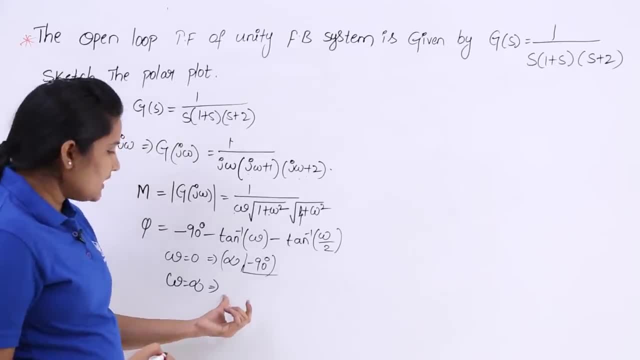 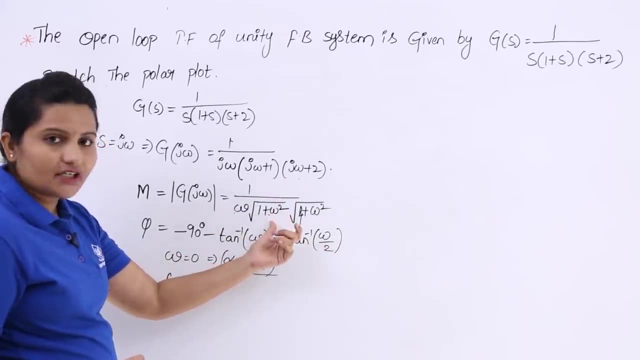 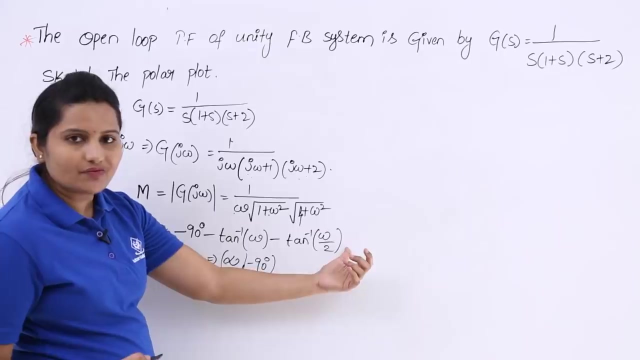 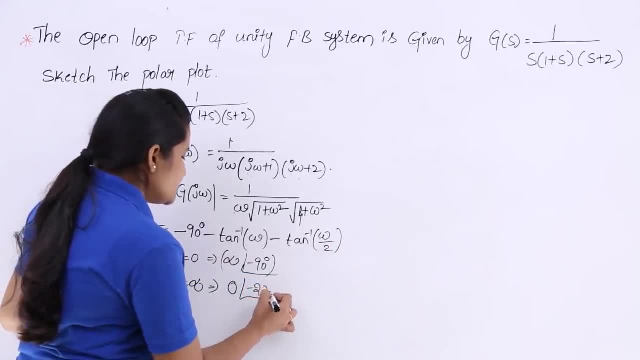 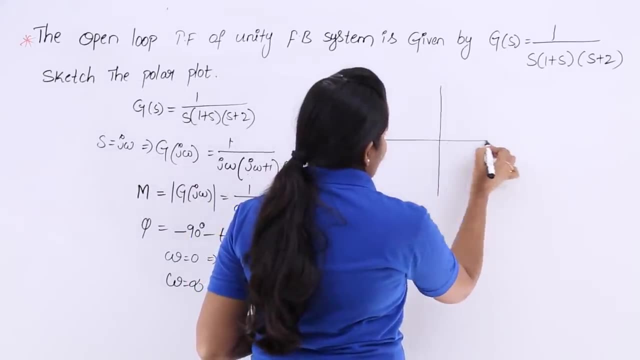 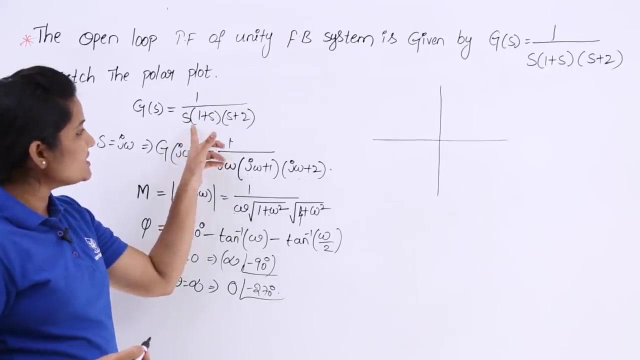 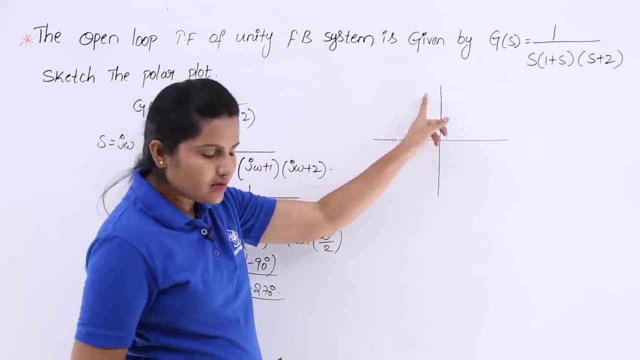 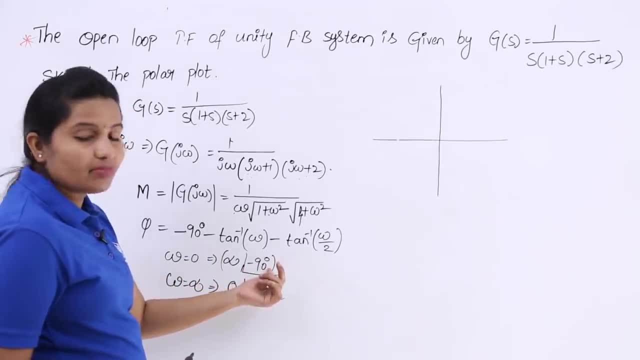 equivalent to 0. you do not know the value, but it will touches minus 90 degrees line. So this is imaginary line, you can see. So omega is equivalent to 0. So omega is equivalent to 0.. So omega is: 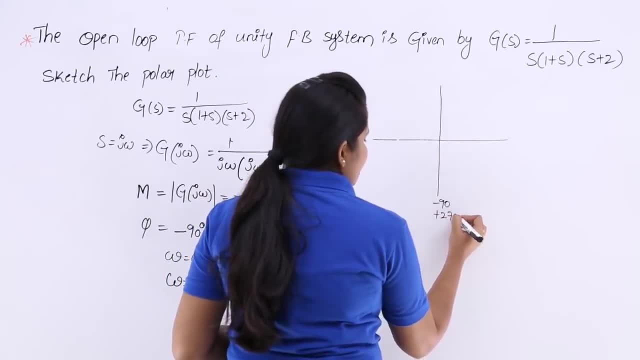 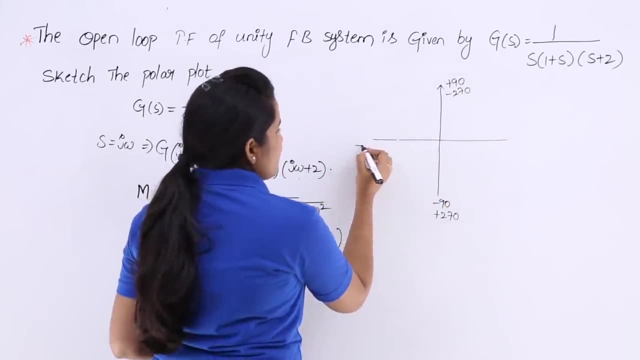 equally 1 by infinity line or negative 0.. So this is negative 90 or negative 0.. Now, this is minus 90 or plus 270. this is plus 90 or minus 270. this is plus 180. this is minus 180.. 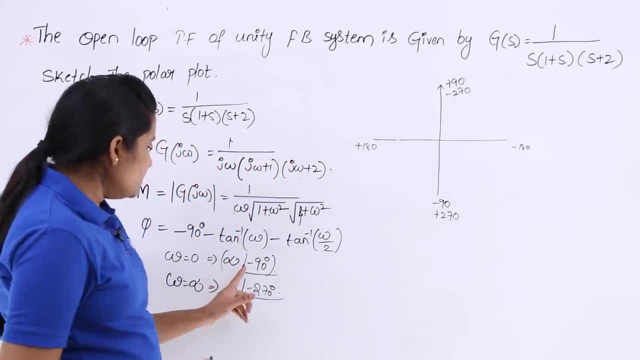 This is 70, but outside a line has an infinity, is relevant the mass minus the mass. For basic interpretation you will be able to see yourself k plus 0, k plus 0. here you are going to see the number of lines behind the glasses etc. For example, this small line here is going: to be 80 k. big line in both these lines will be 90 k. 10 in this, This little bit will be 20, my the small line is equal to 0, and then the growth in the여 Sicherочку, every time former. So it is 90 k, but outside a line this will be 20 k. So what this k will also be. 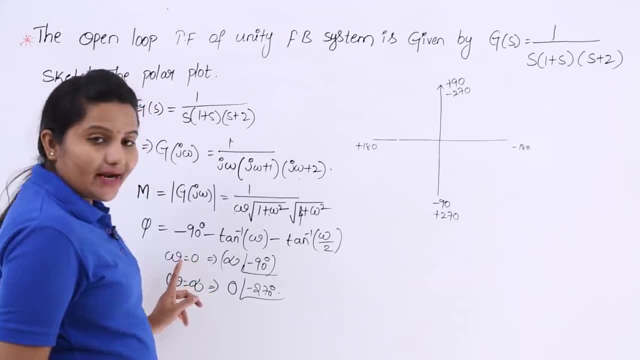 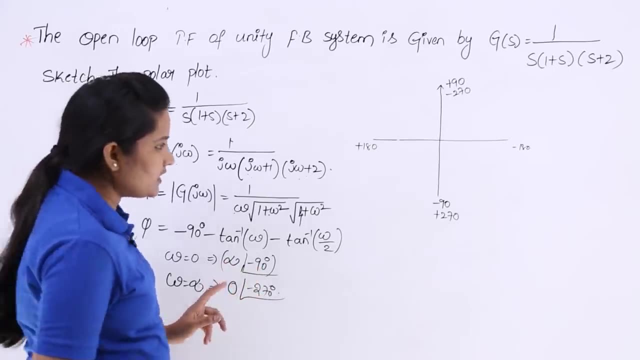 90 k, because what this k is itself is great. because k is negative. 1 by 90 degrees in every. at omega is equivalent to 0, at omega is equivalent to 0. the plot will touch minus 90 degrees line at infinity, So at infinity it will touches, means I do not know where it will touches this line. 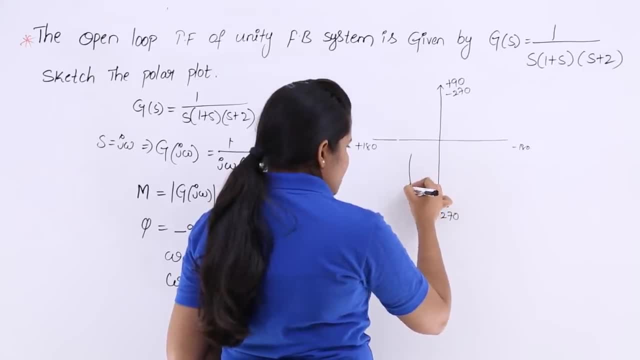 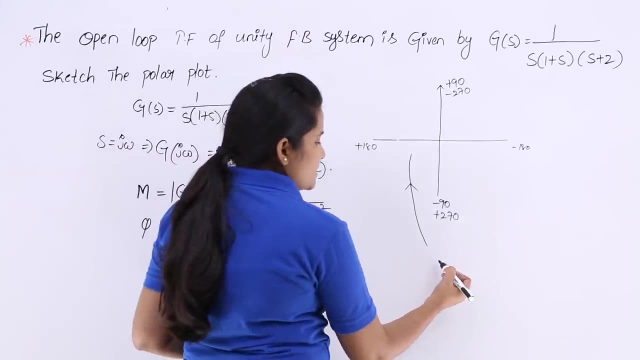 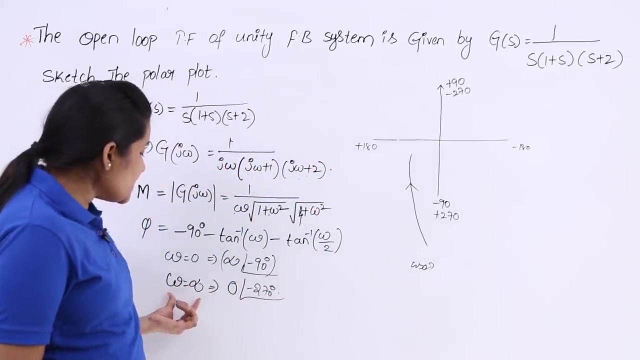 So that is why I am leaving like this. I am leaving like this, So the direction will be like this and, coming to this point, this is some somewhere at omega is equivalent to 0, it will touches. So I do not know where omega is equivalent to 0 and at omega is equivalent to. 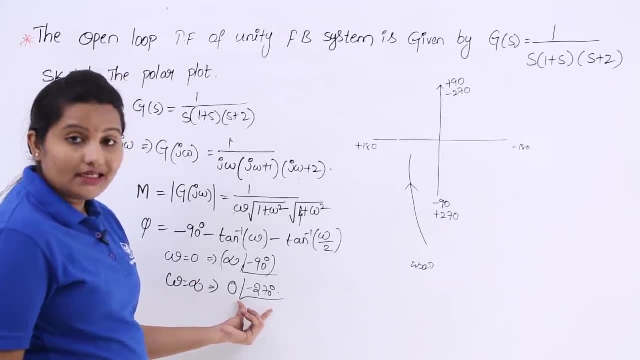 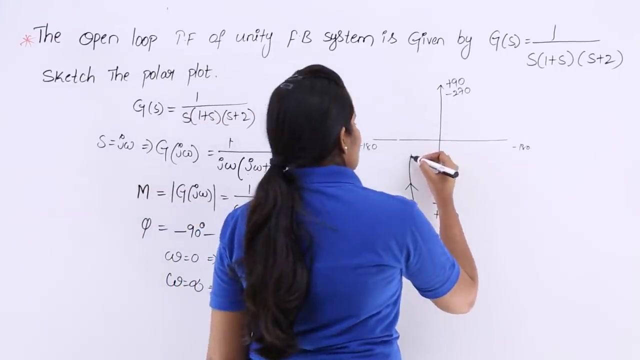 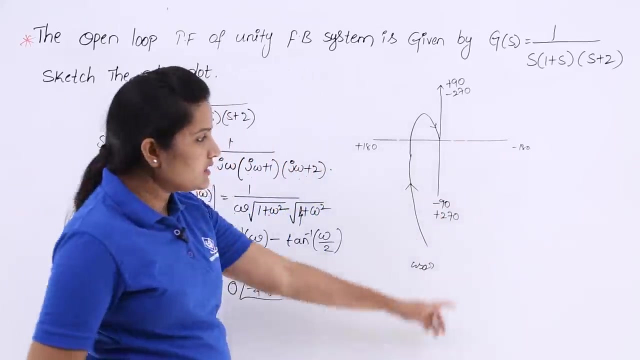 infinity, then here it will touches minus 270 degrees at 0.. So definitely it becomes 0 in 270 degrees means there the frequency is omega is equivalent to infinity. So that means it will touches 270 degrees at 0.. It will touches 270 degrees at 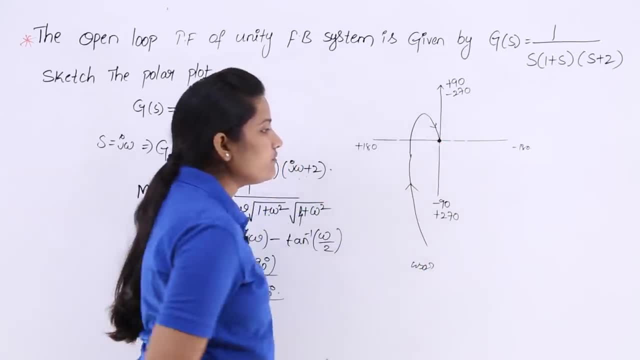 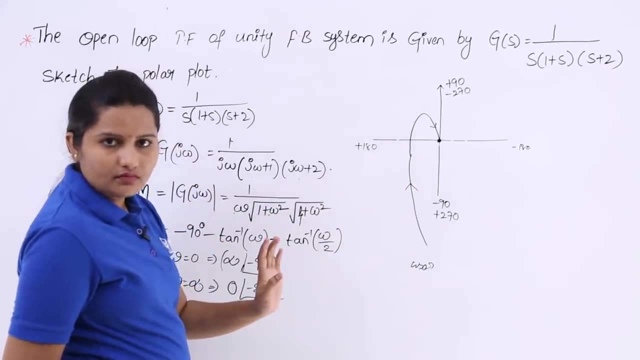 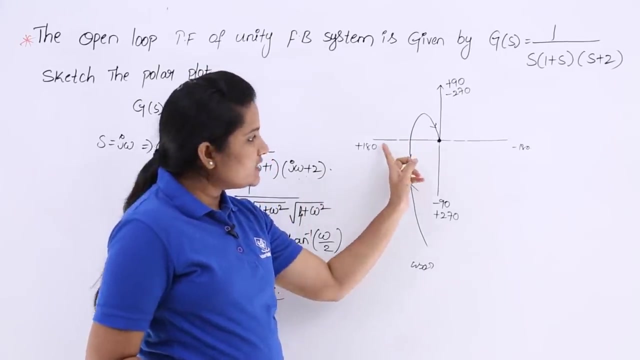 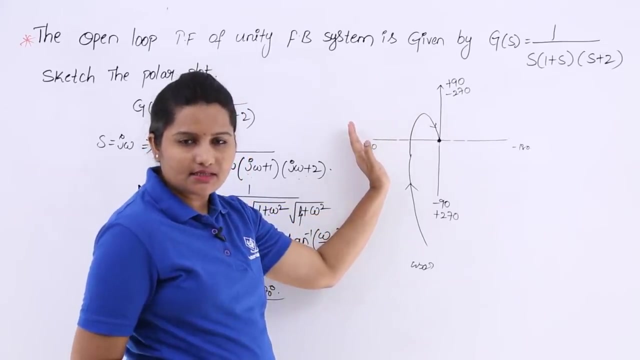 infinity 0,. you can see here at 0.. So now, here you can see this line. this line is interacting with this negative real axis. this is positive real axis and this is negative real axis. This is touching, this plot is touching the negative real axis at 180 degrees. This is 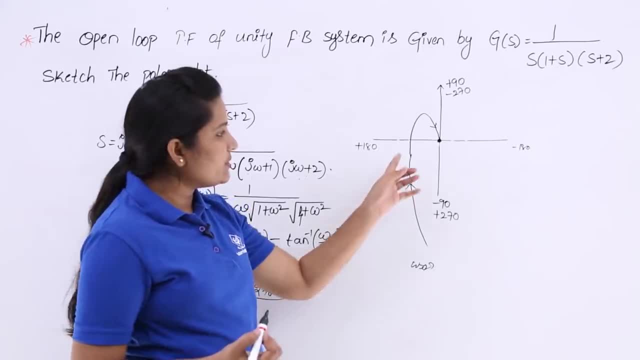 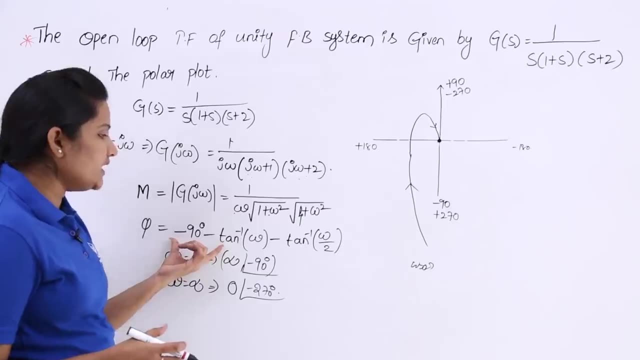 touching negative real axis at 180 degrees. So that means at omega we can substitute. omega is equivalent to 180 degrees in this phase. We can equate 180 degrees to this. If you equate 180 is equivalent to minus 90, minus 10,. 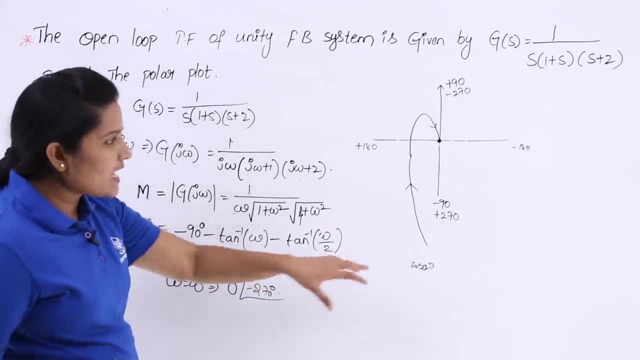 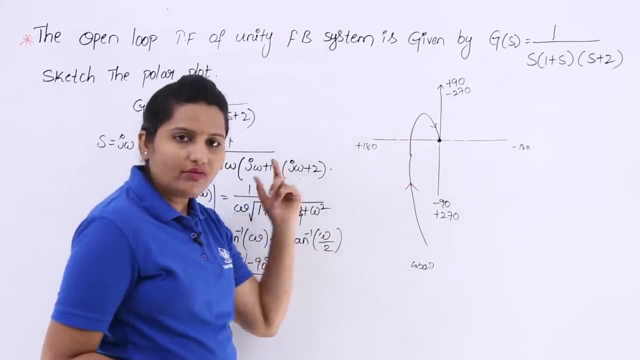 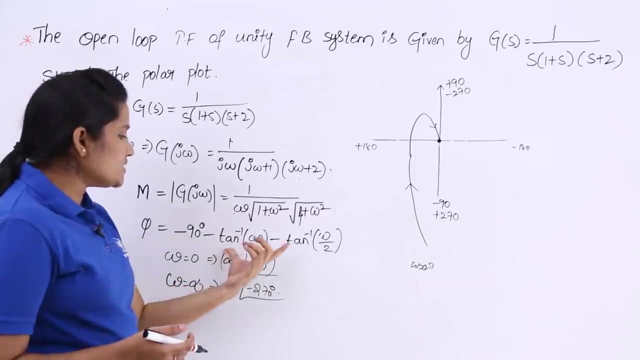 minus 10, inverse omega by 2.. So, as this is interacting with this negative real axis at 180 degrees, you can equate this phase is equivalent to 180 degrees. If you are equating 180 degrees with this, you are going to get omega is equivalent to root 2.. In some other problems, 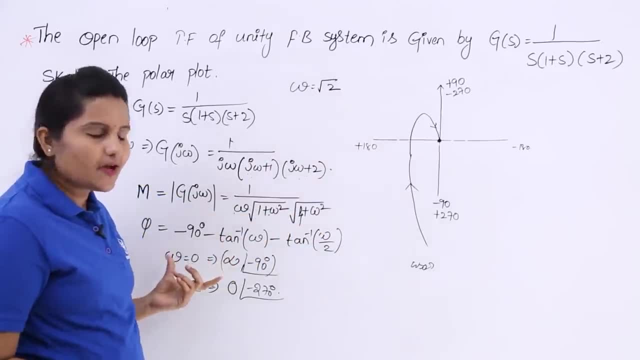 you are going to get some other angle, equivalent to this phi, and you will get omega value. Whatever omega value you are getting and you need to substitute in this, You need to substitute in this means. so here, in magnitude, you need to substitute this omega value. 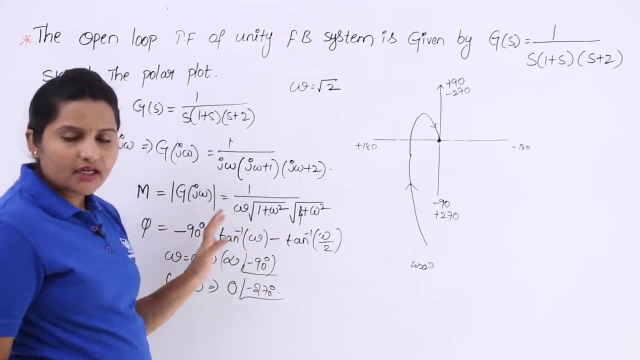 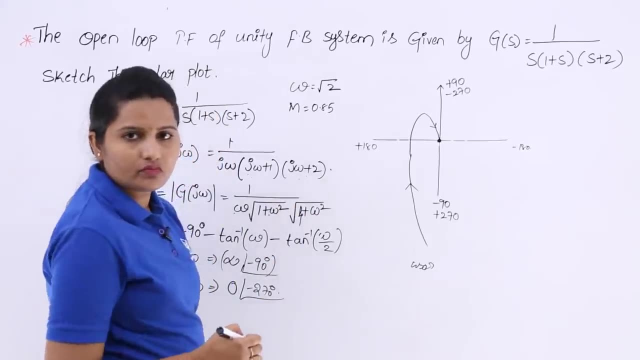 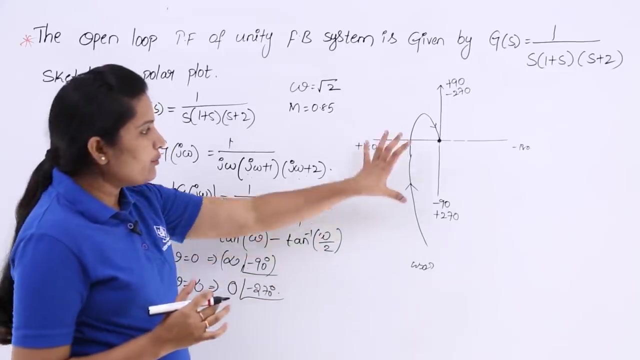 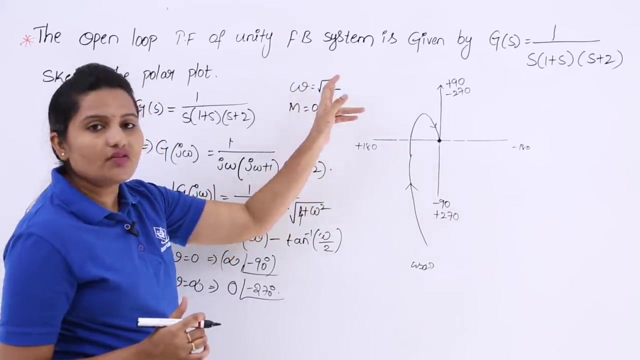 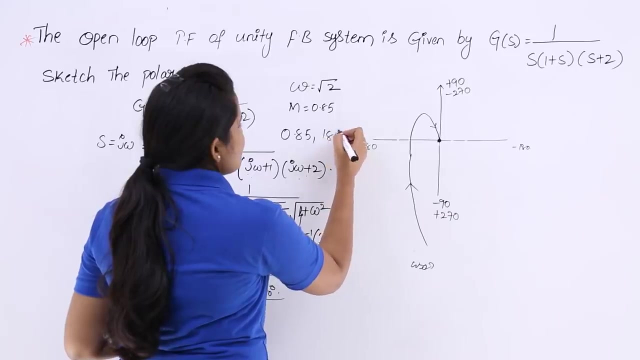 You just substitute: omega is equivalent to root 2 here and you just calculate: the value is nearly 0.85. something Now clear, see, clearly the point is the polar plot is going to interact. the negative real axis at omega is equivalent to root 2 and the polar coordinates are 0.85,180 degrees. 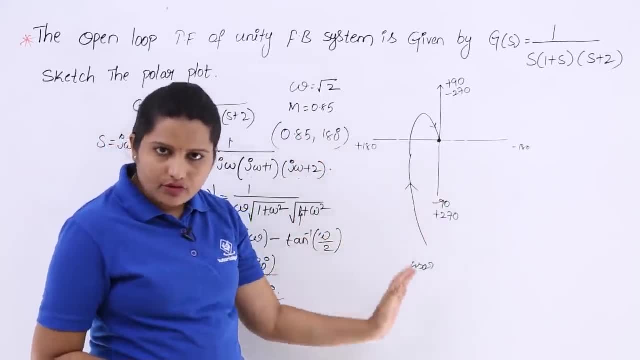 If that is minus 180, you can consider minus 180,. if that is plus 180, you can consider plus 180.. So, whatever the angle your plot is touching, this is a tangent moment, if this angle干个. 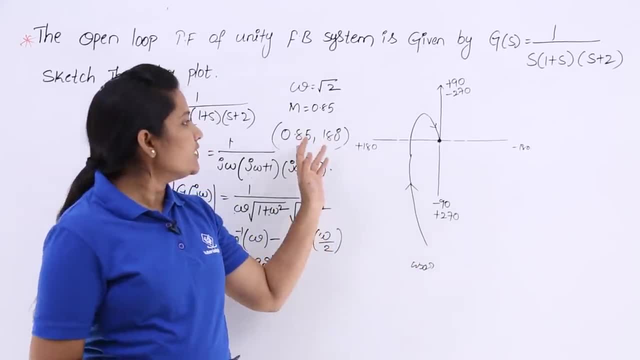 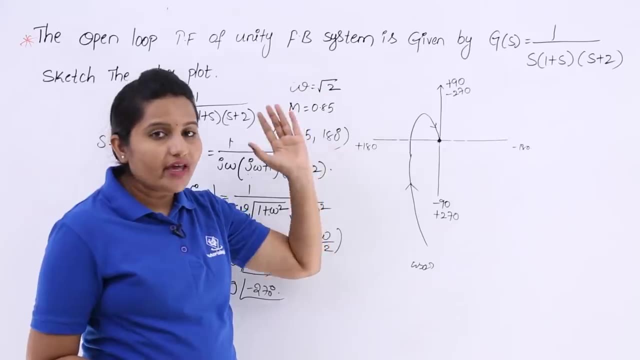 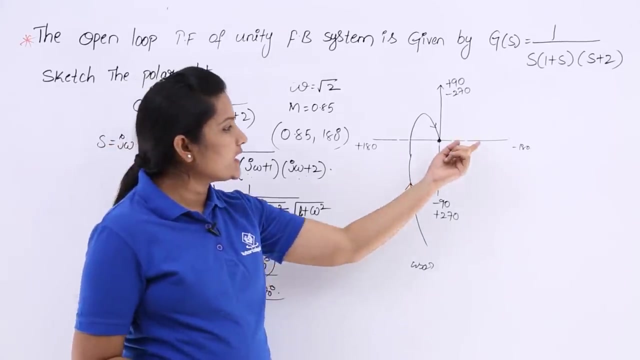 is touching that angle you need to consider. So here this is the meaning. sometimes they will ask like this also: where your polar plot will touches negative real axis. where your polar plot touches negative real axis means so your polar plot is touching or not. first we need to see: yes, it is. 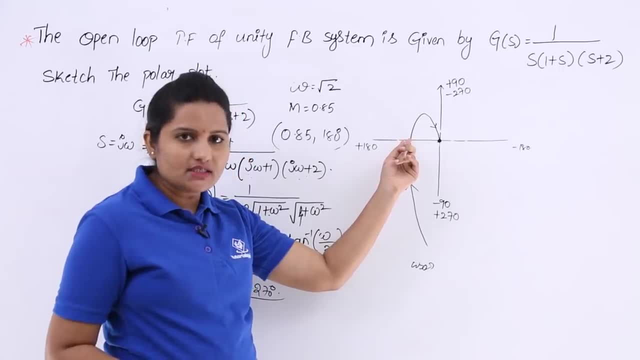 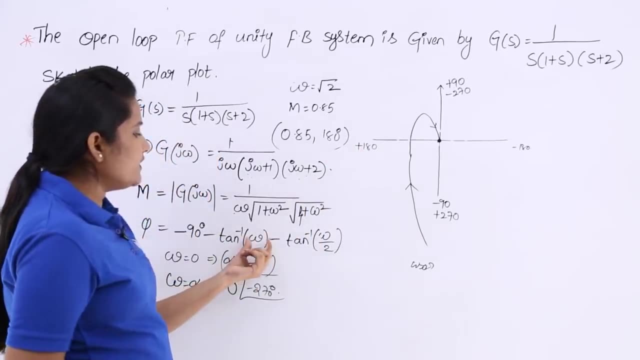 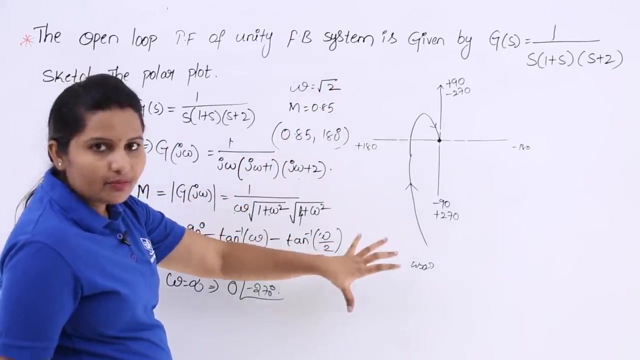 touching negative real axis where it is touching means. so first of all you need to equate this angle with this face so you will get omega value at. value of omega is equivalent to root 2. your polar plot is going to touch here. omega is keep on increasing from 0 to infinity at 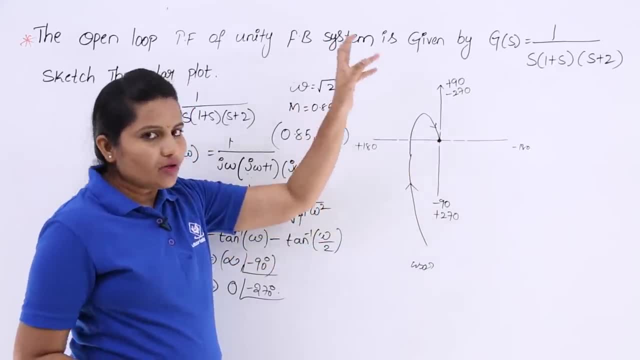 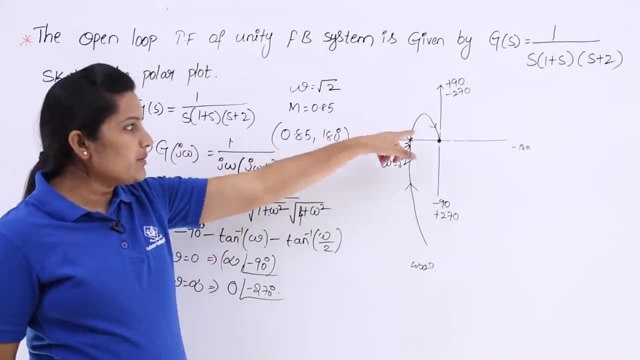 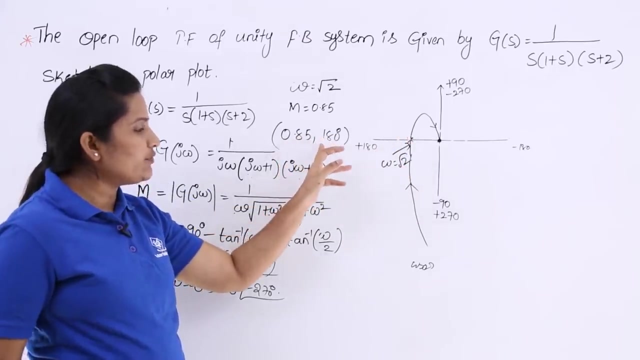 infinity. this will be 0 when omega is equivalent to root 2. this is the point at omega is equivalent to root 2. at this point your polar plot is going to touch this negative real axis. the coordinates of this point is 0.85 comma 180 degrees. So like this we need to draw. 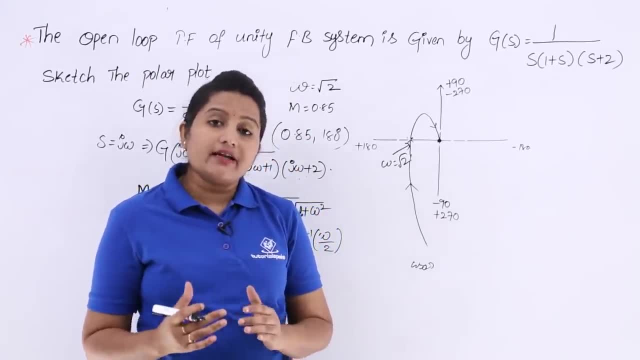 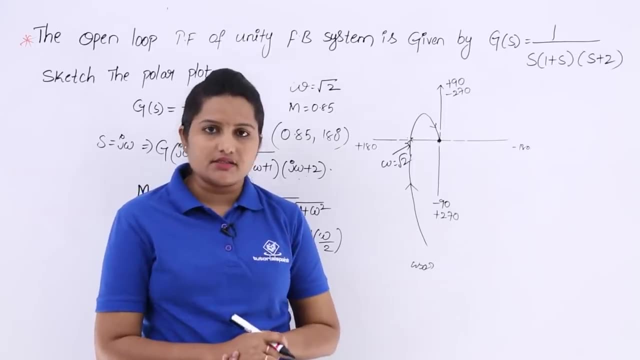 polar plot and we can mention at which frequency, at which frequency your polar plot is touching real or imaginary axis.